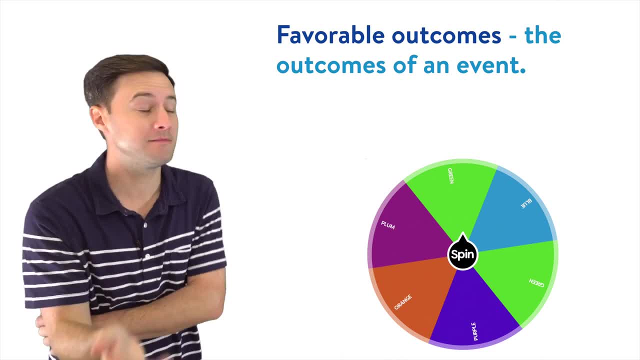 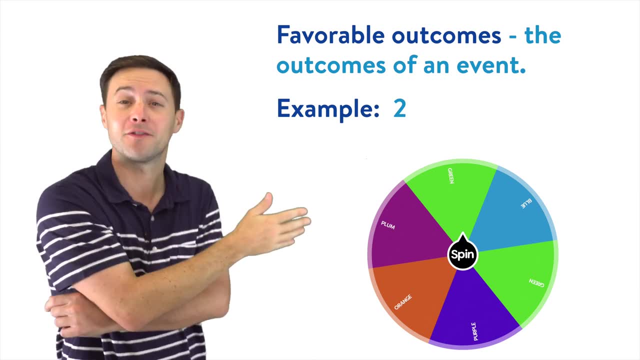 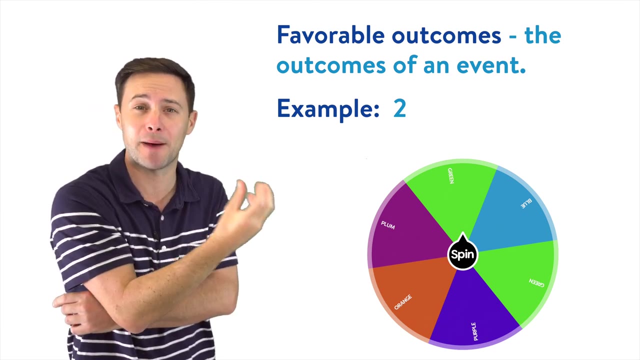 outcomes. So, if the event is to land on green, how many favorable outcomes are there? Well, in this situation there's two, because there are two ways to land on green, which is what we wanted. Favorable outcomes is what you want to happen. How many ways can that thing happen? Now that we 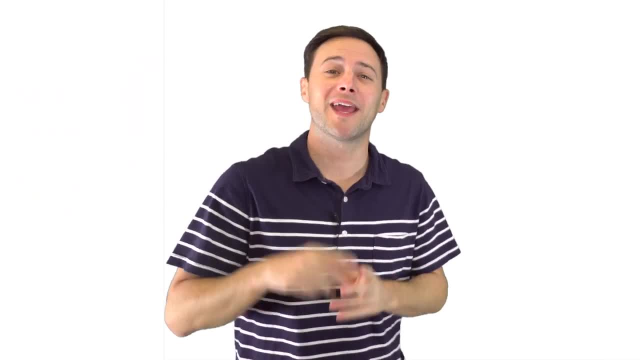 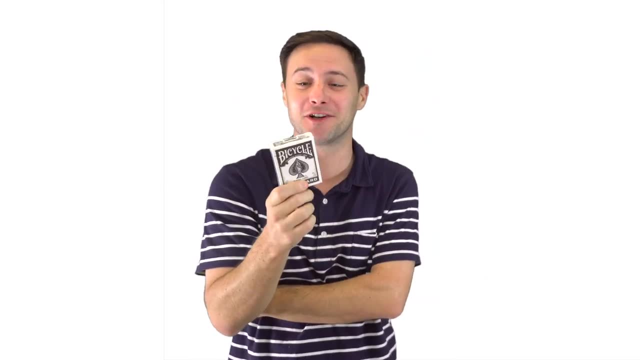 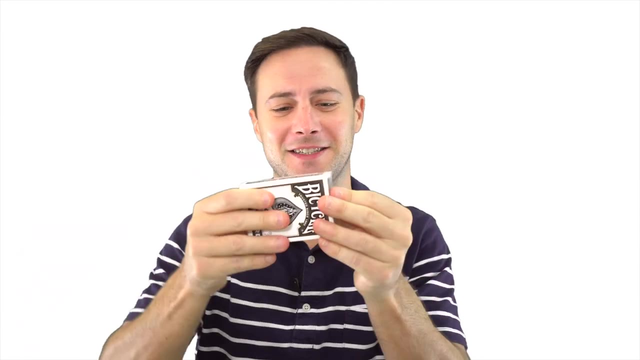 know some new terms. let's get to our first example. All right, example one: you pick a random card from a full deck, All right. well, before we get to this example, I guess we should learn a little bit about cards. This is a standard deck of playing cards. Brand new deck- get rid of. 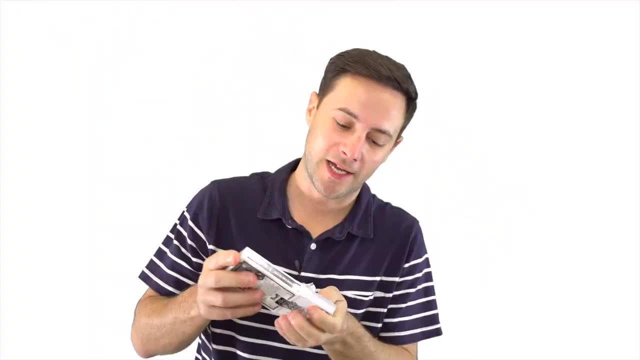 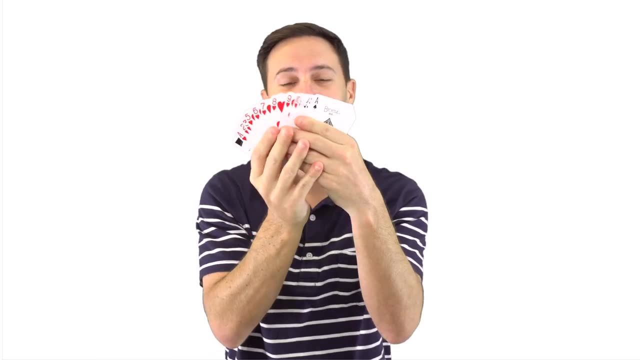 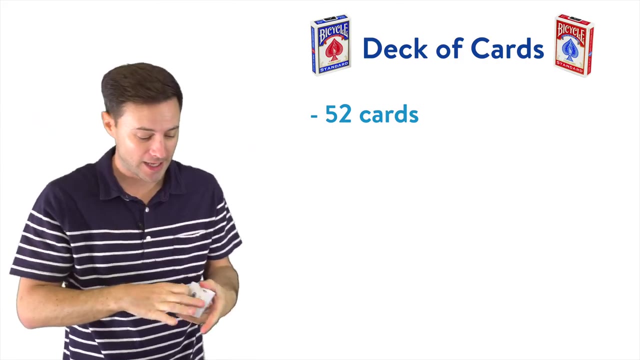 all that. Cut that open, Take out all the cards. Don't need that anymore. So when we talk about a full deck of cards, this is what we are talking about. So first let's break it down. There are 52 total cards in a full deck. 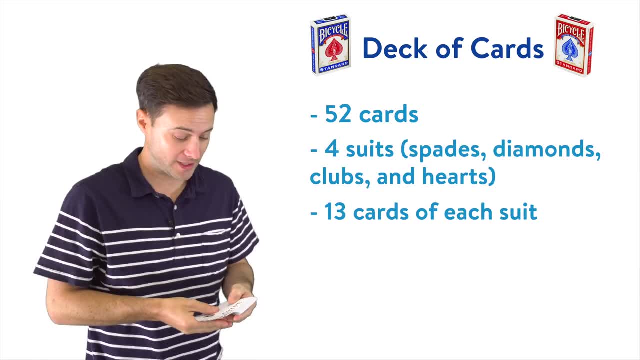 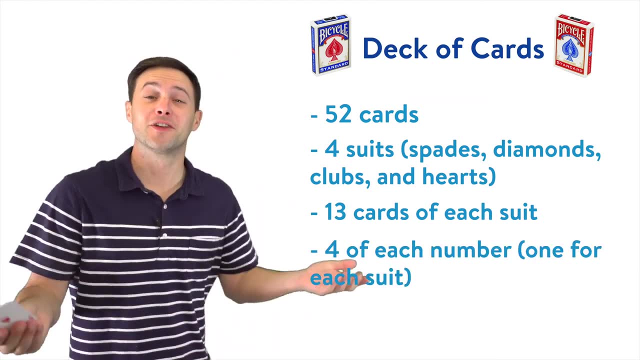 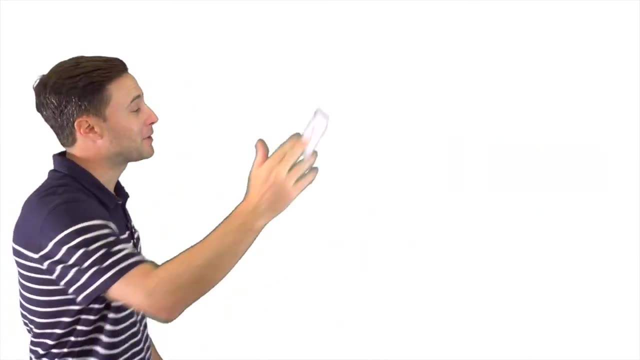 Those 52 cards are broken up into four suits, and those suits are the spades, the diamonds, the clubs and finally the hearts, And so, naturally, there's four of each number. There are four aces, one of each suit. So now, hopefully, you know a little bit something about playing cards. 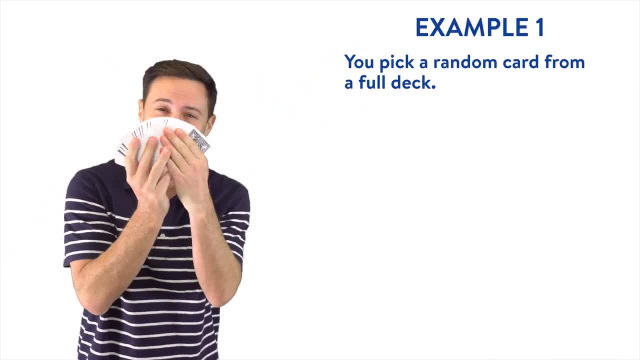 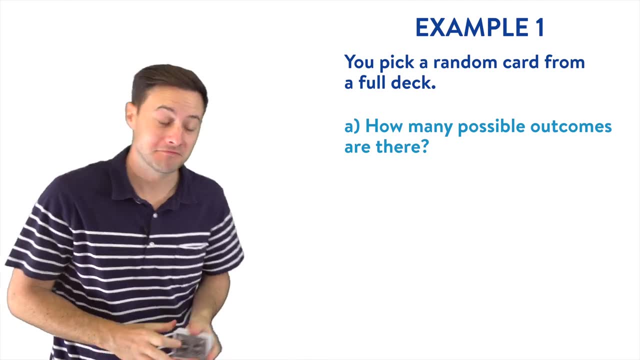 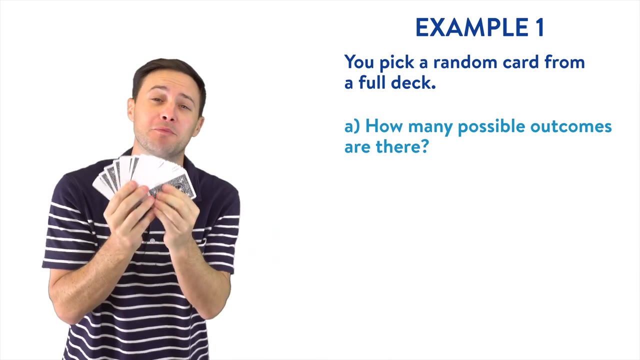 Let's get to the first question. Okay, so we are picking a random card from a full deck, like we said before. So first question is: how many possible outcomes are there? Well, how many cards are there? Right, Each one is equally as likely to get chosen. So how many playing cards are there? 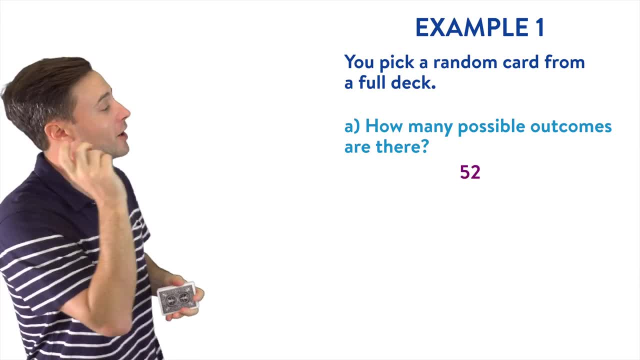 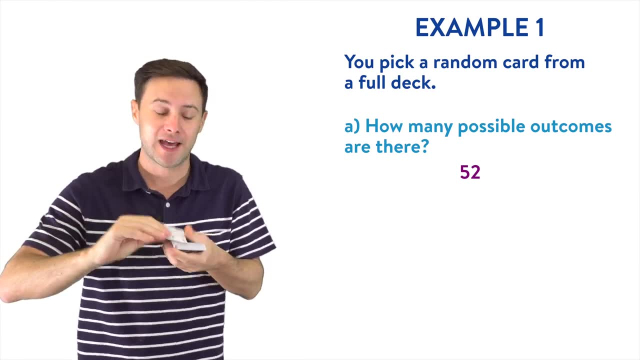 And the answer to that, if you remember, is 52.. So there are 52 total possible outcomes. If we wanted to list each possible outcome, we would have to list cards. So we would say: ace of clubs, two of clubs, three of clubs, four of clubs. Those are all the. 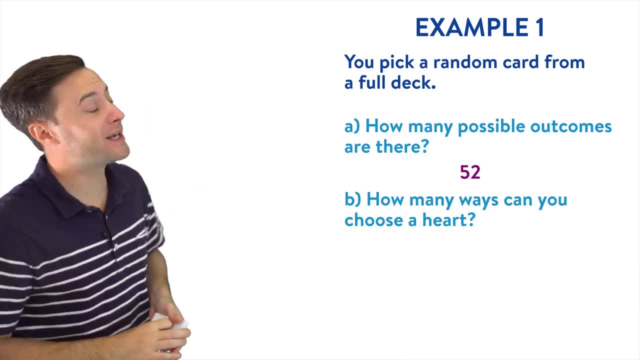 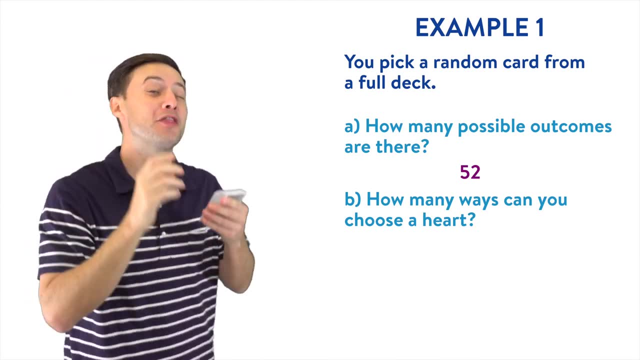 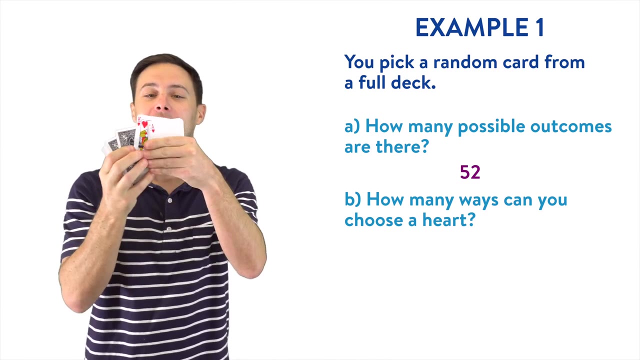 possible outcomes, All right. question B: How many possible ways can you choose a heart? Well, if you remember, heart is one of the four suits and there are 13 hearts, or 13 of every suit in a deck. So, if we look, every single one of these would be a way to choose a heart, right?